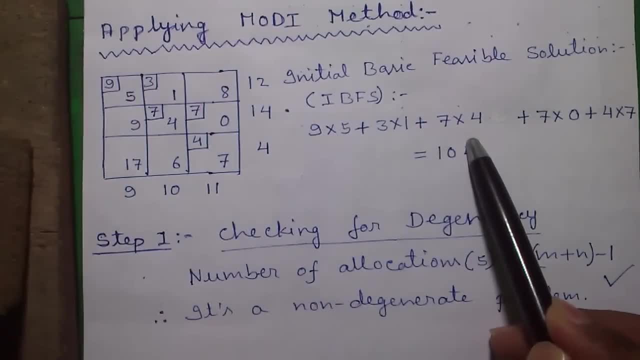 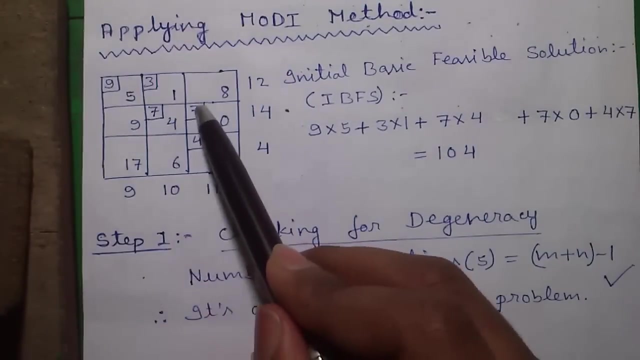 This value was found by North West Corner Rule And we will check whether we can reduce the cost by Modi method or not. So step 1.: Checking for degeneracy. The number of allocations is 5.. 1,, 2,, 3,, 4, 5 allocations. 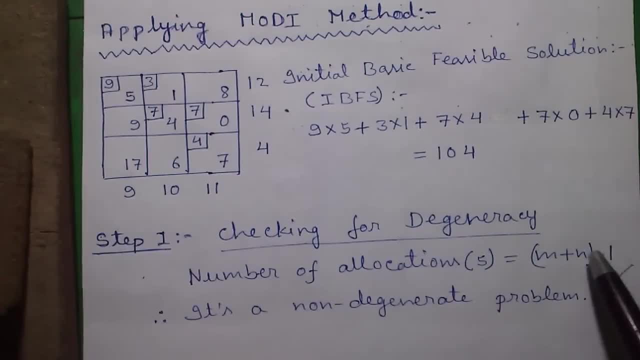 Equals to, or not, m plus n minus 1.. Where m is the number of rows is 3 and n is the number of columns, which is 3.. So the number of allocations is 3 plus 3 minus 1.. That is 5.. 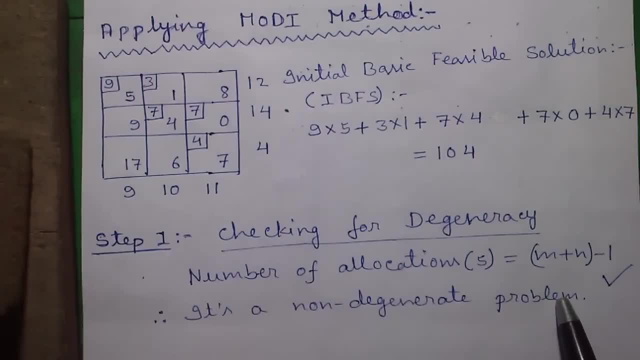 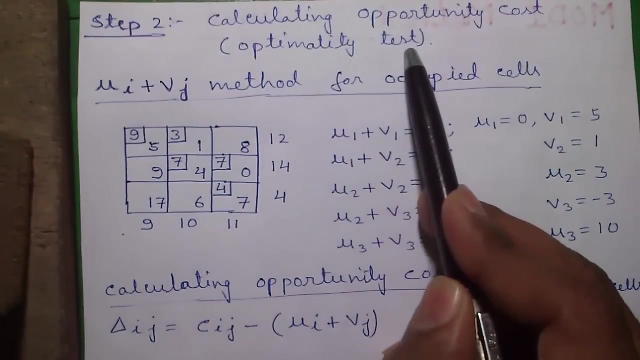 So it is a non-degenerate problem If the number of allocations is greater or lesser than m plus n minus 1. That is called a degenerate problem. There is a special technique for solving them. So for now, step 2. Doing the optimality test. 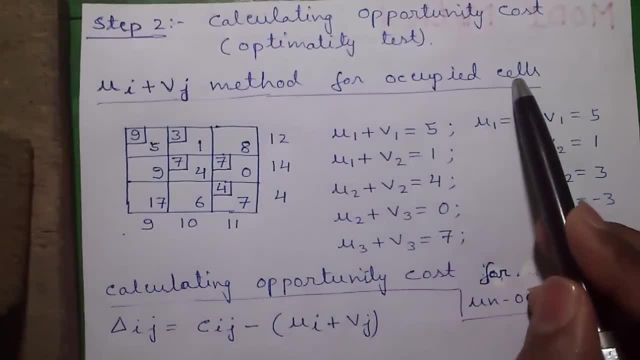 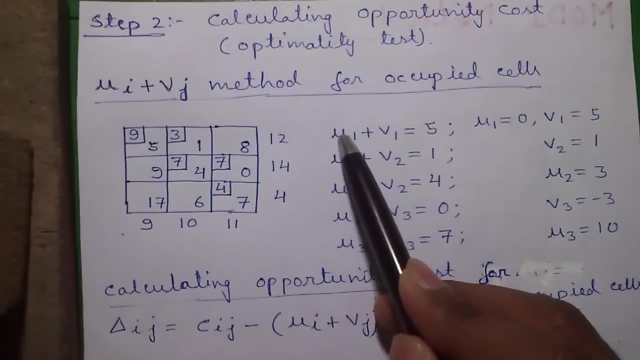 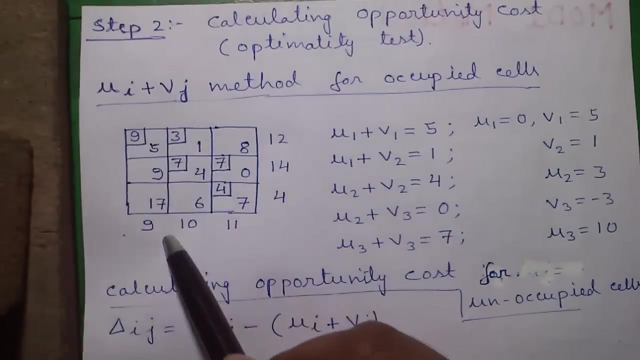 First the Ui plus Vj method for occupied cells or allocated cells, Also called the basic cells. U represents the row number and V represents the column number. That means U1 in row 1 plus V1 is column 1. The cell value is 5.. 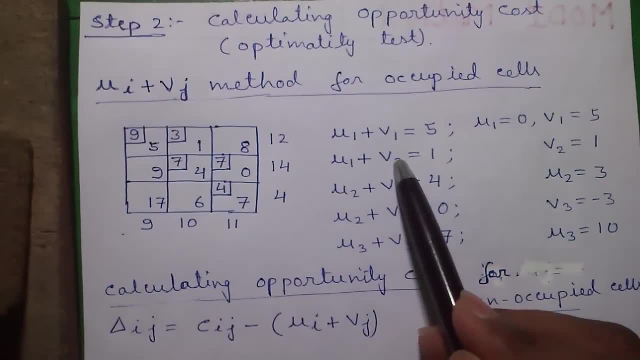 Similarly in U1 plus V2.. Row 1, column 2.. The cell value is 1.. U2 plus V1 equals to 4.. U2 plus V3 equals to 0. And U3 plus V3 equals to 7.. 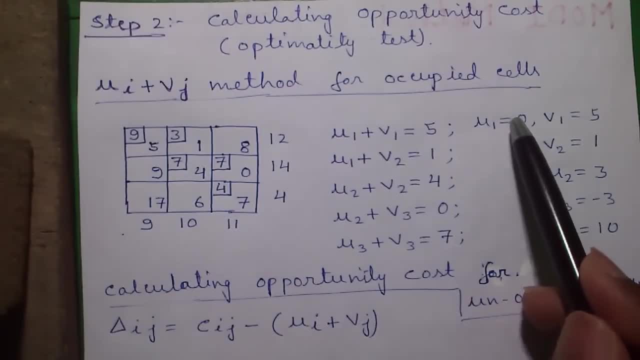 Let's take: U1 equals to 0. So that gives us V1 equals to 5.. Similarly, if U1 is 0.. V2 equals to 1.. And if V2 equals to 1. Then U2 equals to 4 minus 1, 3.. 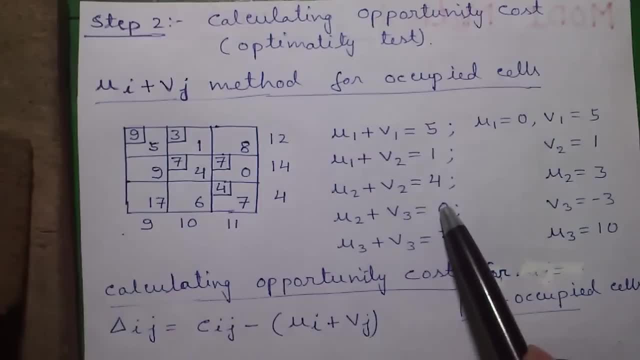 And if U2 is 3. Then V3 equals to 0 minus 3, minus 3.. And if V3 equals to minus 3. Then U3 equals to 7 minus of minus 3. That is, U3 equals to plus 10.. 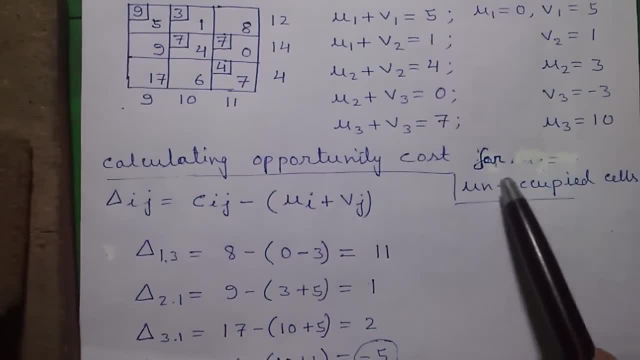 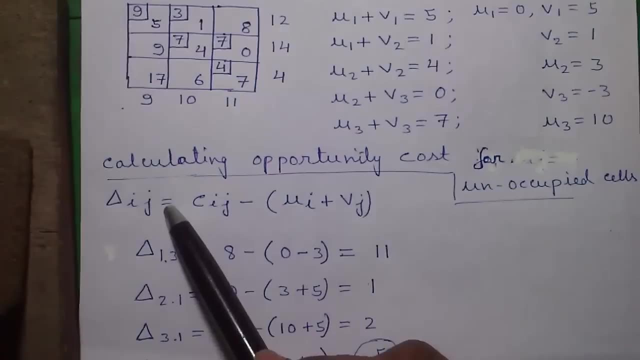 Next, calculating the opportunity cost for unoccupied cells, Also called non-basic cells, Which is given by Del: ij equals to Cij minus Ui plus Vj. Again, U and V represents the rows, Row number and column number, And Cij represents the cell value. 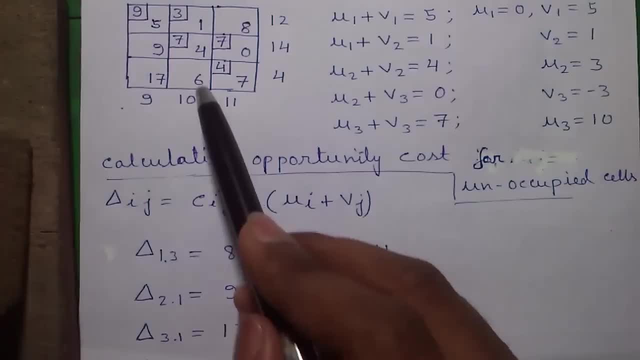 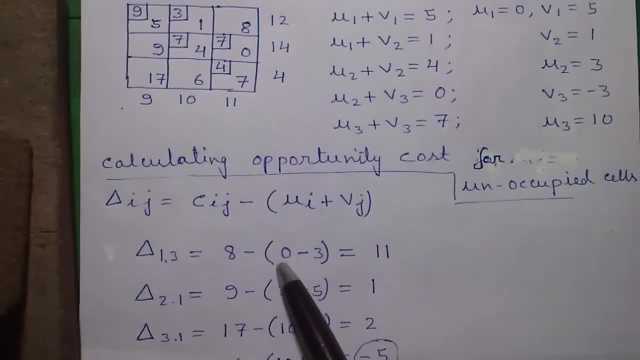 So del 1: 3. That means in row 1, column 3. The value is 8 minus U1 is 0.. Plus Vj is or V3 is Minus 3.. So that gives us 8 minus 0, plus minus 3.. 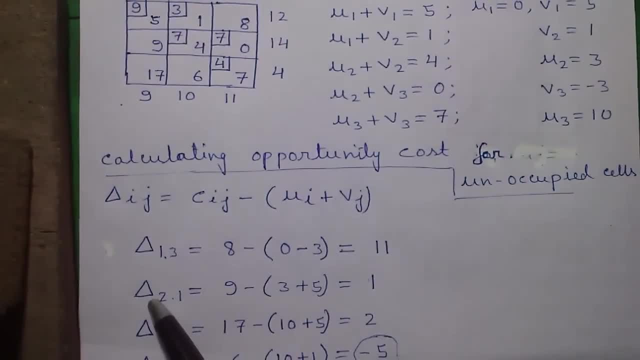 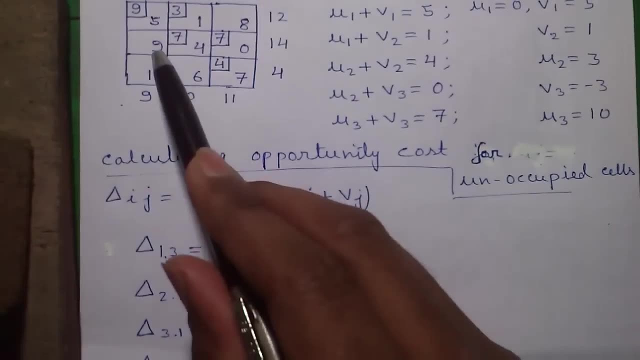 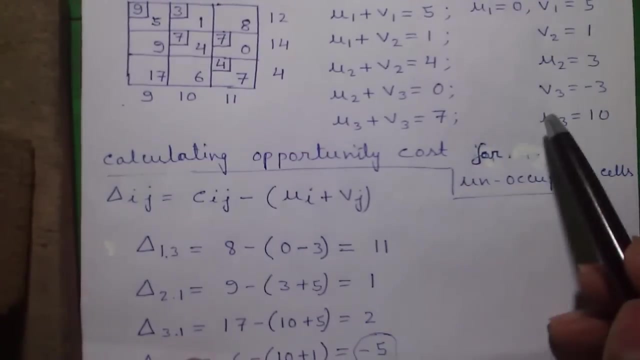 Which is plus 11.. Similarly for del 2, dot 1. That means in row 2, column 1. The value is 9 minus U2 is plus 3.. Plus V1.. V1 is plus 5.. That gives us 9 minus 8.. 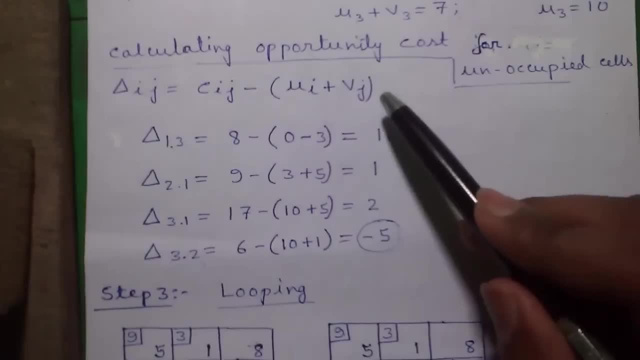 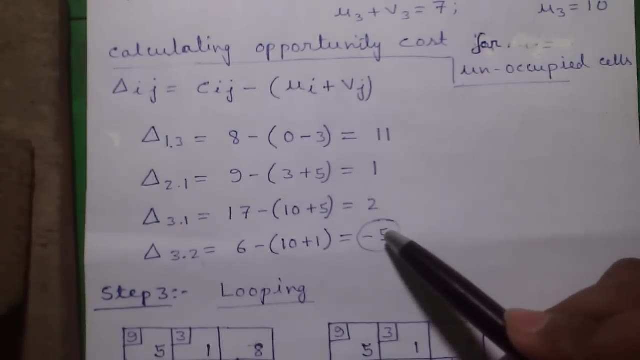 That gives us 8 equals to 1.. So calculate the opportunity cost For each of the unoccupied cells And check whether the values are greater than or equal to 0.. Or less than 0.. The rule is If all the values are greater than 0. 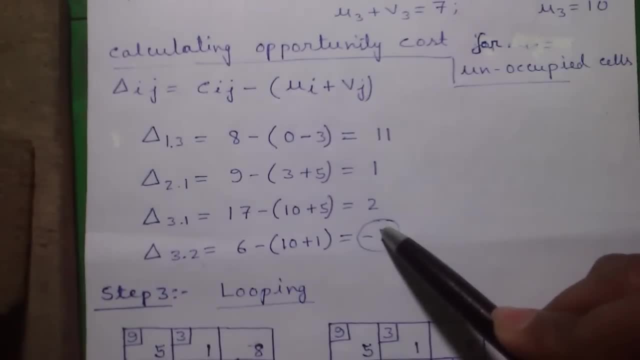 Then the current solution is both optimal and unique. And if all the values are greater than 0. With at least one value as equals to 0. Then the solution is optimal but not unique. And if there is at least one negative value. 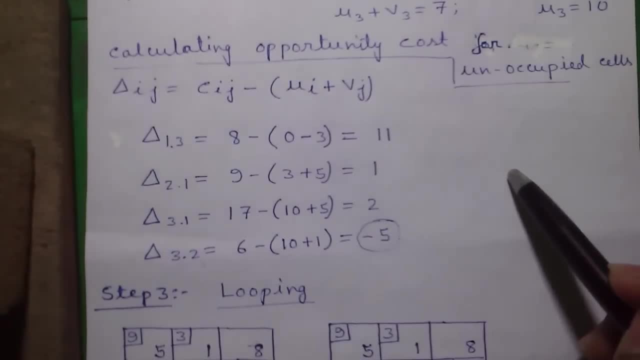 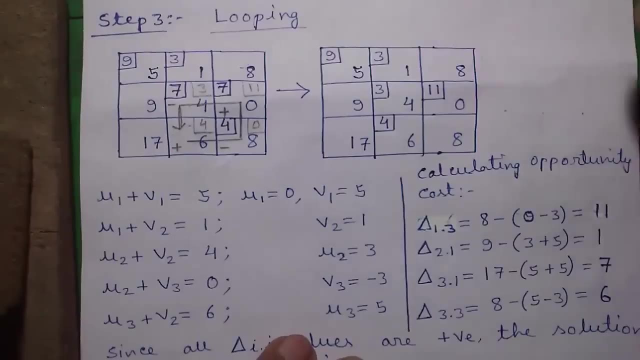 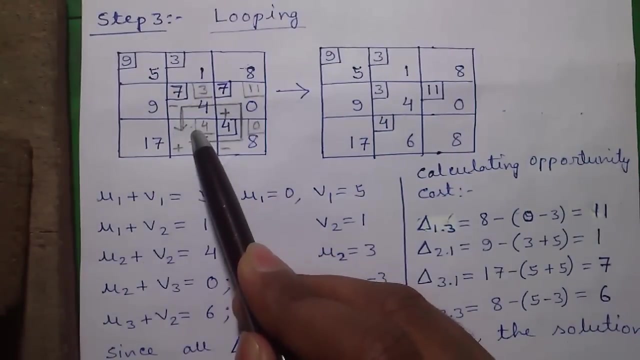 Then the solution is neither optimal nor unique. So here our present allocation solution is neither optimal nor unique. To get the optimal solution We have to do the looping and reallocation. This is called a loop. There are some rules for looping, Rule 1. 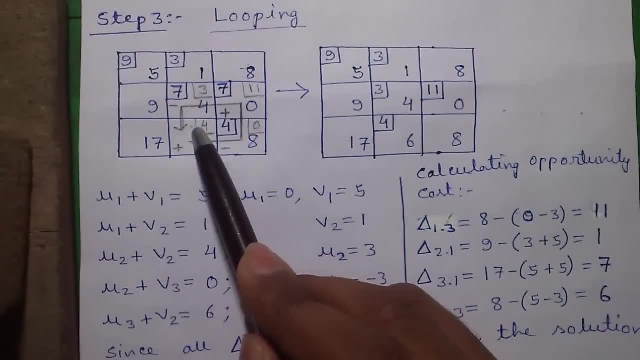 The loop must be a closed loop. That means the starting cell and the ending cell of the loop Must be the same cell- Rule 2.. The starting and the ending point of the loop Must be an unoccupied cell- Rule 3.. 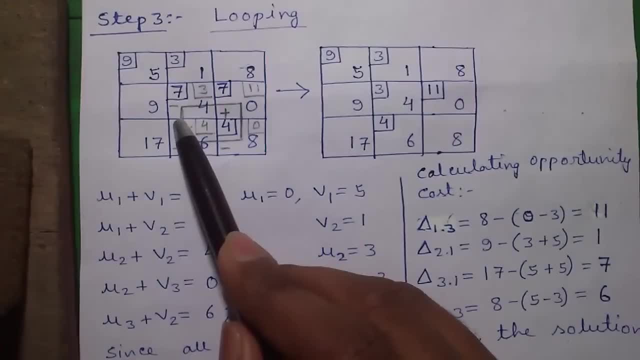 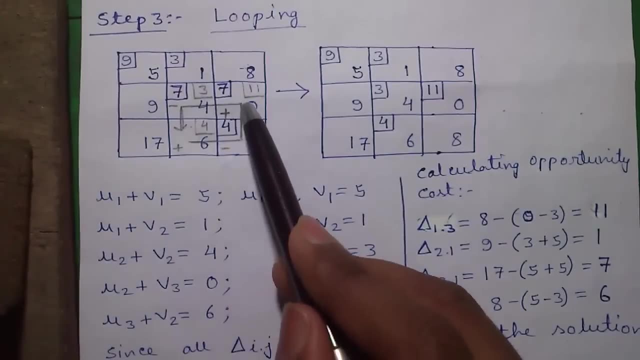 The loop may take any path, But at each corner points of the loop That must be an occupied cell. Here, at three corner points, We have three occupied cells. Next we will find out the smallest value Among all the allocated values in loops. path. 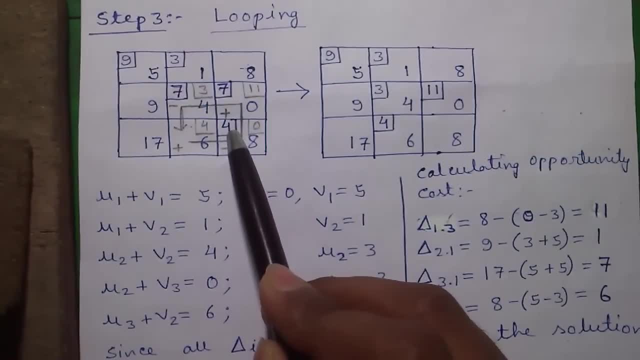 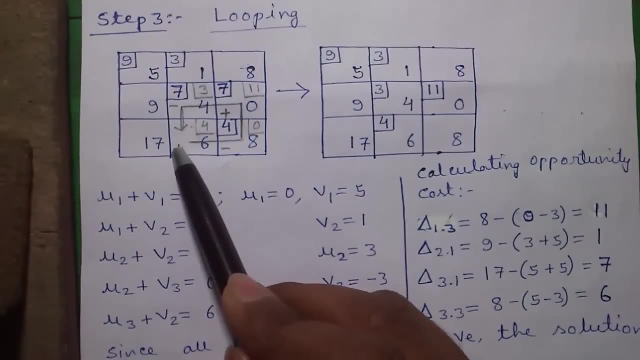 Here we have 7,, 7 and 4 as allocated values, And the 4 is the smallest value. Next we will mark our first cell as plus cell, Next cell as minus cell, Next cell as plus cell And next cell as minus cell. 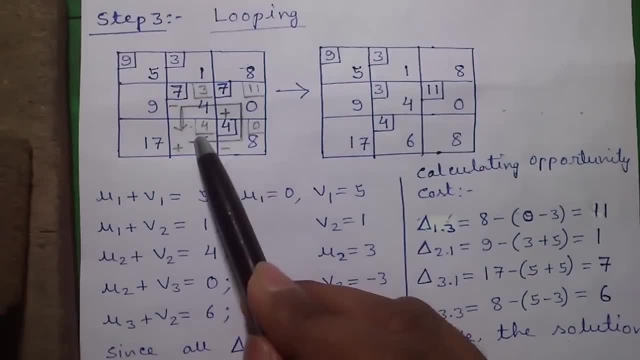 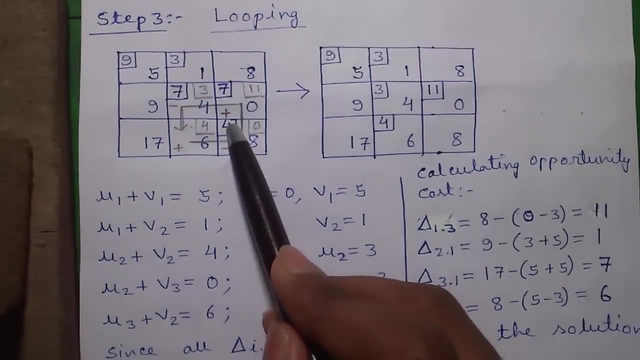 That is in alternative order Along with the path of the loop. Our smallest value is 4.. We will plus or allocate that value in the first cell, So our first allocation is 4.. In the next cell is the minus cell, So we will subtract 4 from the allocated value. 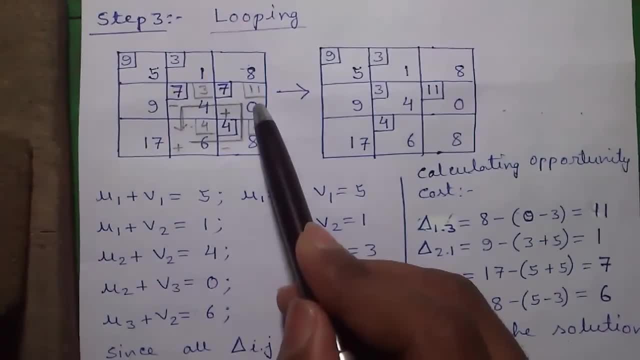 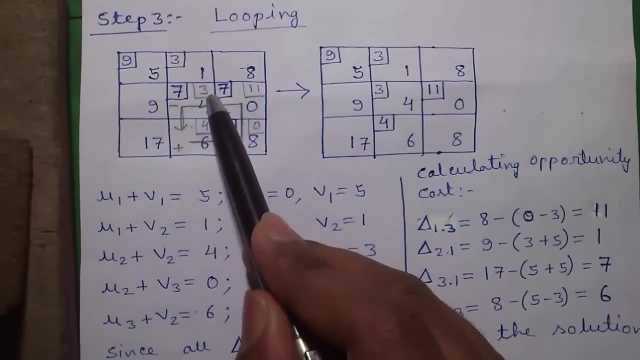 So 4 minus 4 is 0.. Next cell is a plus cell. 7 plus 4 equals to 11.. Next cell is the minus cell. 7 minus 4 is the 3. So we have got our newly allocated matrix. 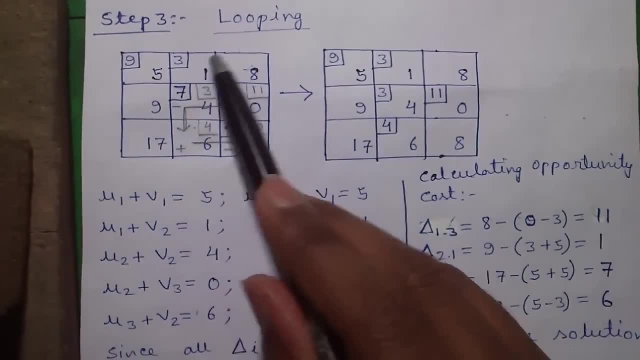 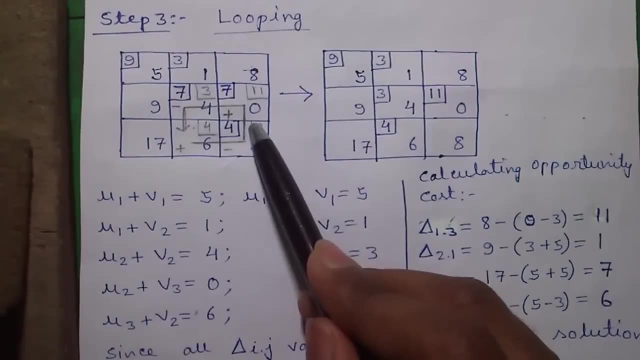 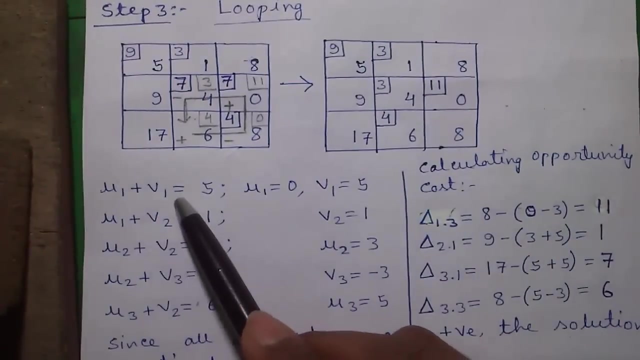 So writing this, We get 9,, 3, same as previous- 3,, 11 and 4. And this 0 means no allocation. Again, on this newly allocated matrix, We will do the Ui plus Vj operation And the opportunity cost calculation. 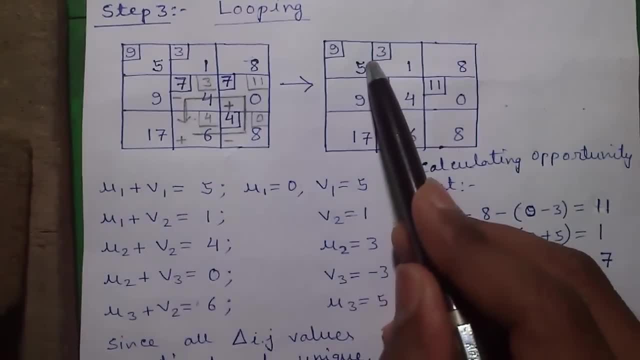 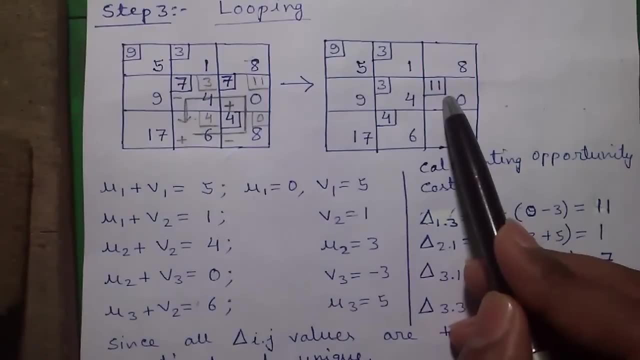 So that gives us: U1 plus V1 is 5. U1 plus V2 is 1. U2 plus V2 is 4. U2 plus V3 is 0. And U3 plus V2 is 1.. 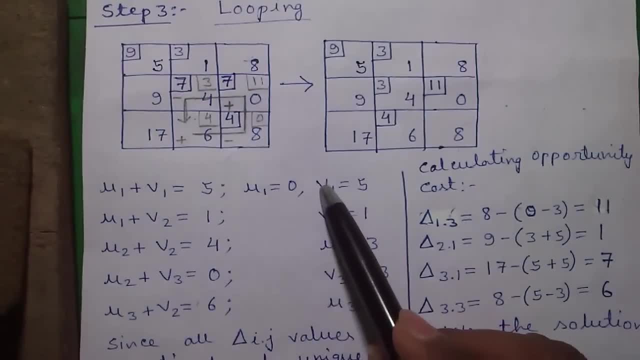 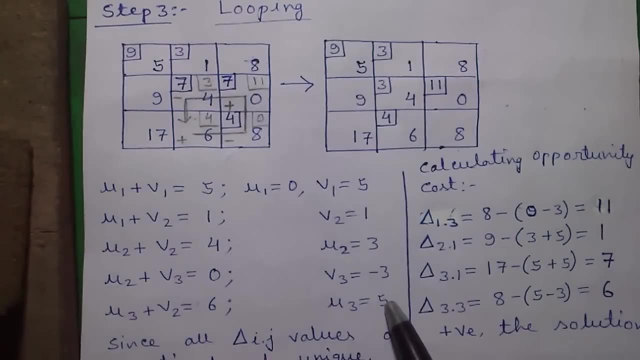 U3 plus V2 is 6. So that gives us V1 equals to 5., V2 equals to 1., U2 equals to 3., V3 equals to minus 3. And U3 equals to plus 5.. 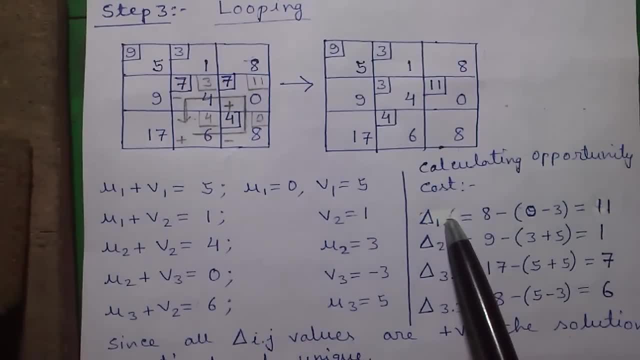 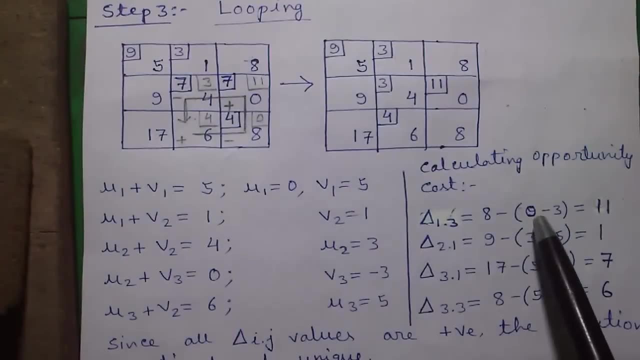 Next calculating opportunity cost: Del 13 is 8 minus U1 plus V3.. That is plus 11.. Del 2.1.. The value is 9 minus U2 plus V1 plus 5.. That is plus 1.. 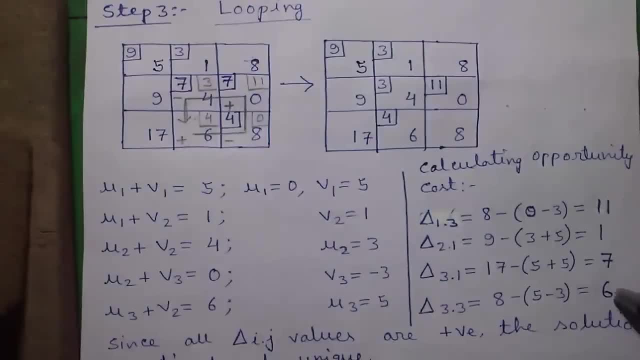 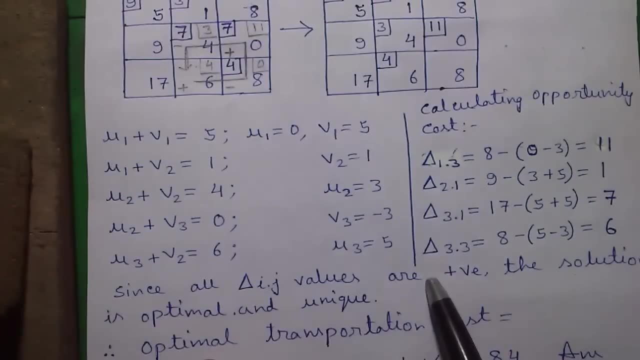 So do the opportunity cost calculation, as previous, And you will see, this time all the values are positive. Since all the del ij values are positive, Then the solution is optimal and unique. Unique means there is not an alternate solution to this problem. That means this solution is optimal and final. 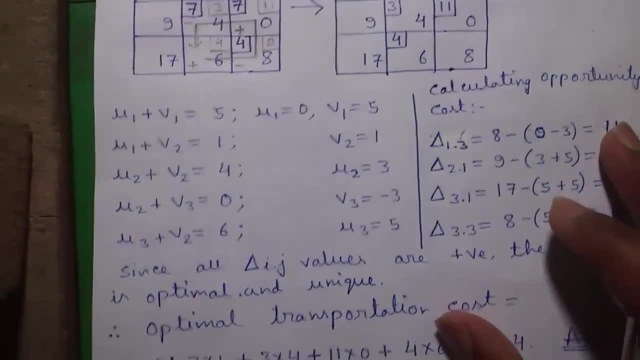 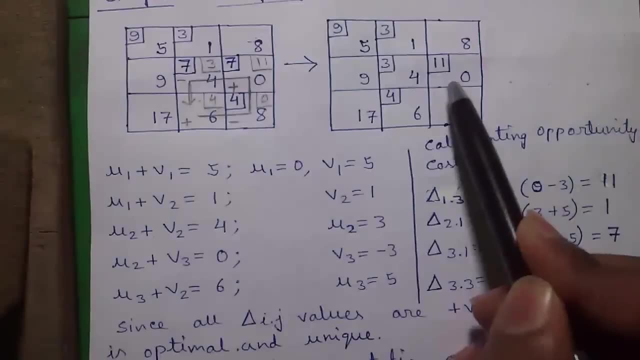 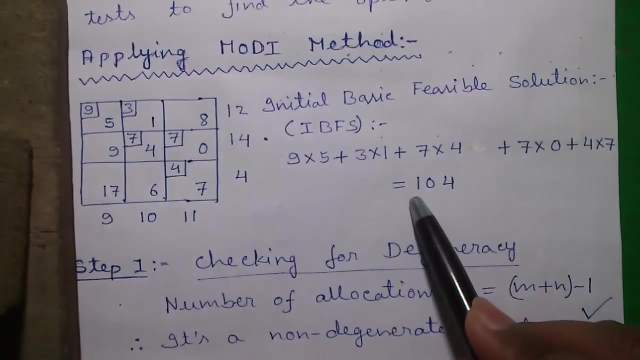 Next, calculating the optimal transportation cost Which is given by the previous technique: 9 into 5 plus 3 into 1 plus 3 into 4 plus 11 into 0 plus 4 into 6. Which is 84. Previously it was 104 units. 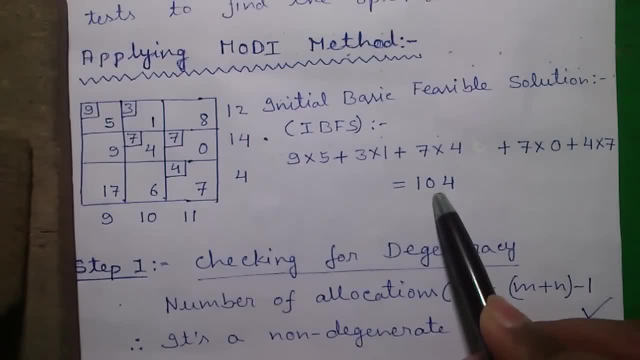 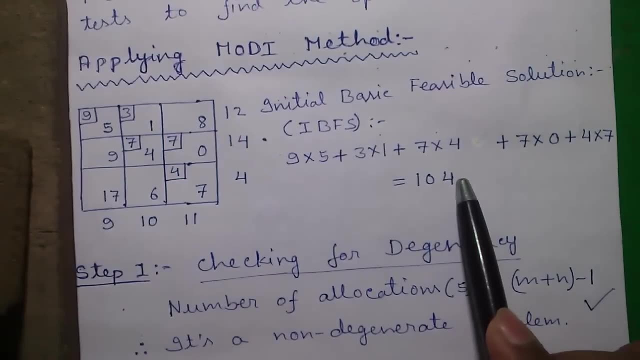 So we have reduced our cost of transportation by 20 units by Modi method. So, friends, this was my video On Modi method. Hope this video was helpful to you. If you like the video, Please like it And subscribe to my YouTube channel. 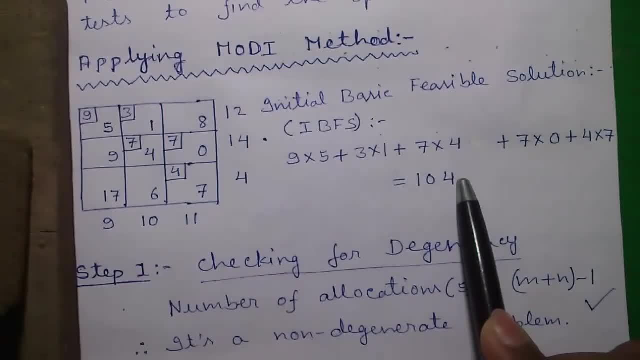 By subscribing, you can stay connected with me And get regular updates from me, And please share the video on your YouTube, Google Plus, Facebook and Twitter accounts. By sharing the knowledge, you may help someone else. I have uploaded some other videos on operation research. 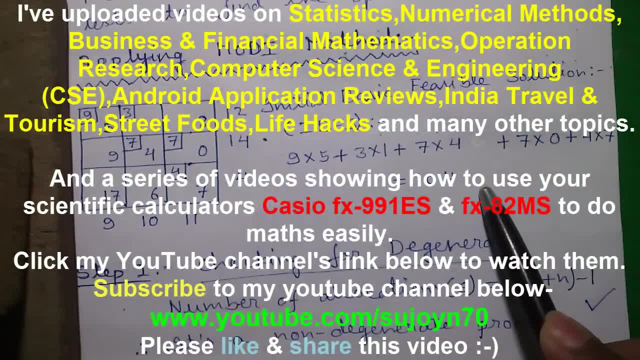 On Vogel's approximation method, Northwest corner rule Matrix, minimum method, Assignment problem, etc. The link to my operation research playlist is given in the video description. Click that to watch all my operation research videos. Apart from operation research, I have uploaded some videos on statistics. 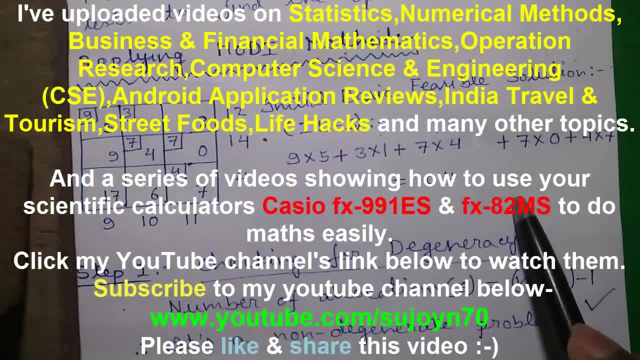 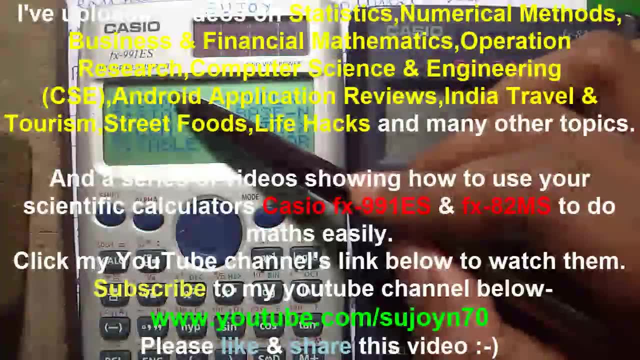 Probability, Numerical methods, Number systems, Computer science and engineering, etc. And some exciting videos on this Casio FX99ES calculator, From mode 1 to mode 8 of this calculator, To how to use all the modes of this calculator. 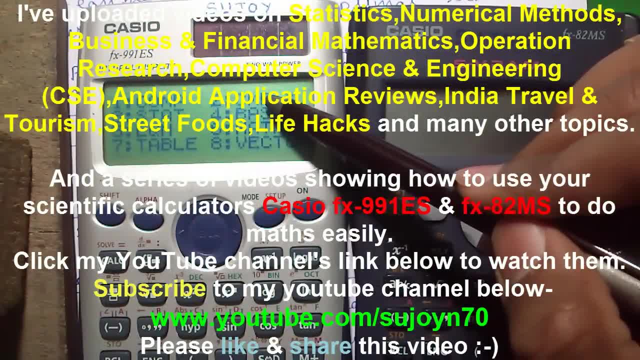 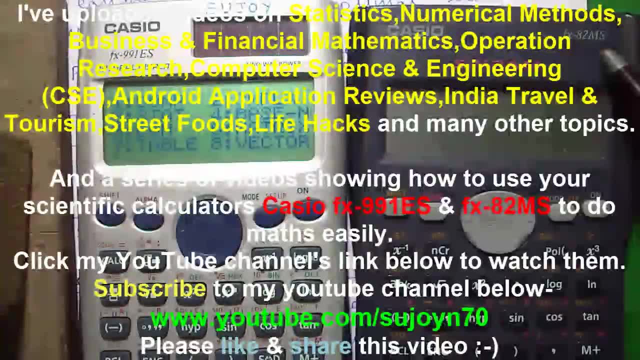 To do math quickly and easily During exams. Also, some videos on this Casio FX82MS calculator. Like 20 cool features of this FX82MS calculator: Finding standard deviation or linear regression on this calculator, Calculating trapezoidal rule, etc. 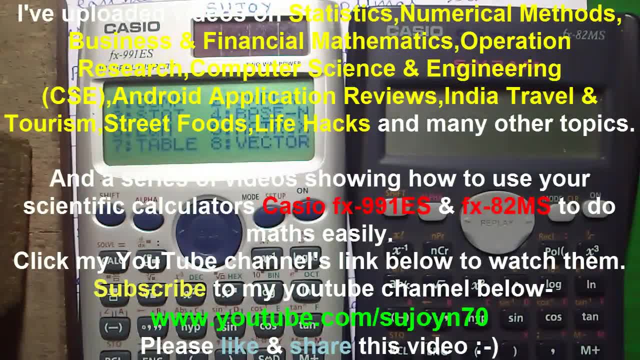 So thanks for watching, See you in my next video And stay connected by subscribing.